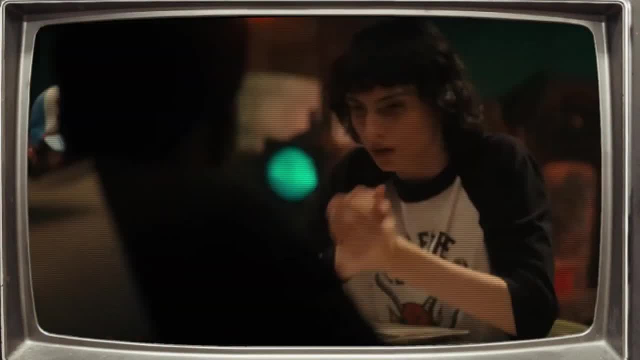 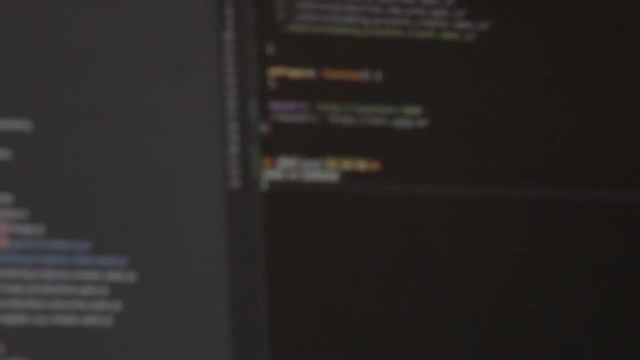 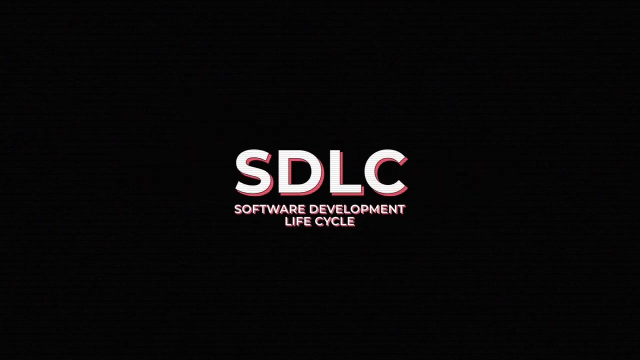 How do you decide what your next step on a project is? Let's hope you're not relying on a roll of the dice, especially when the decision concerns something as costly as software development. In that case, we suggest a tried-and-true method like the Software Development Life Cycle or SDLC. It's a standardized process that describes different stages of building high-quality software. 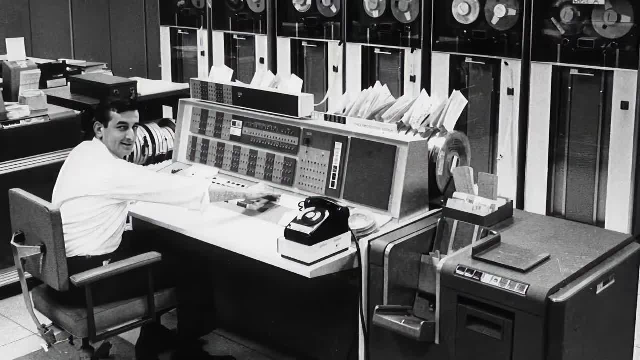 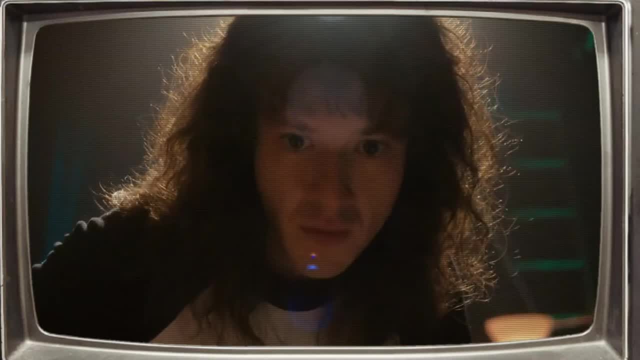 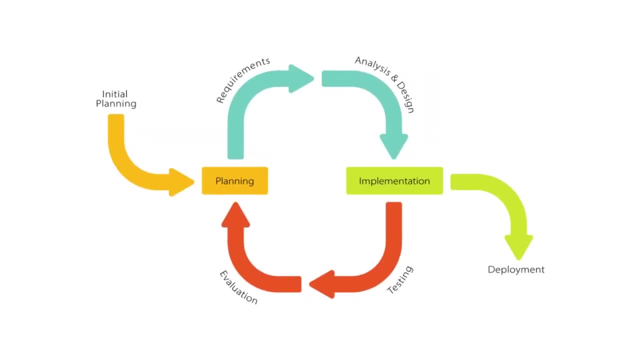 SDLC was conceived in the 1970s as a way of formulating the development of large-scale business systems, but it prevails today as a reminder of what stages a product goes through on the way to eventual- we hope- success. There are many methodologies addressing this sequence of stages that you might have heard of, So today we will talk about the phases of SDLC and the methodologies applying them. 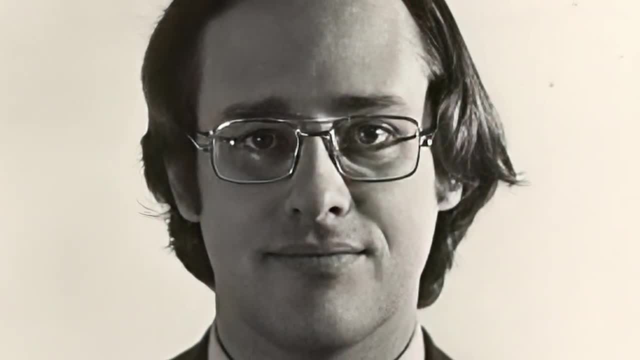 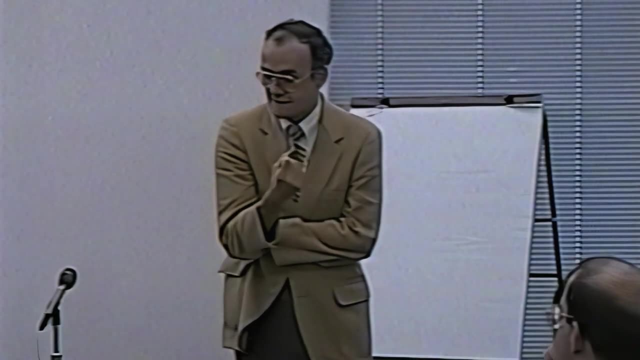 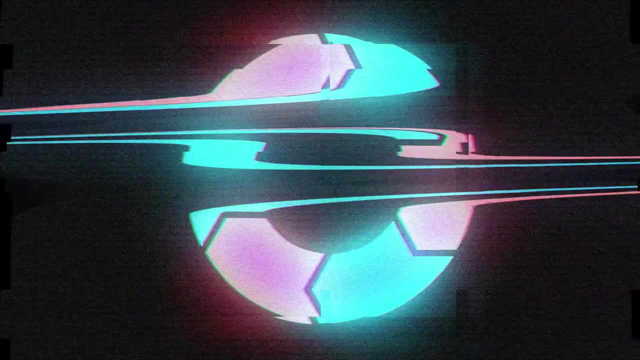 The father of the Software Development Life Cycle was a computer scientist and a director at Lockheed Software Technology Center in Austin, Winston W Royce. In his influential article Managing the Development of Large Software Systems, he described implementation steps that are similar to what we use today. 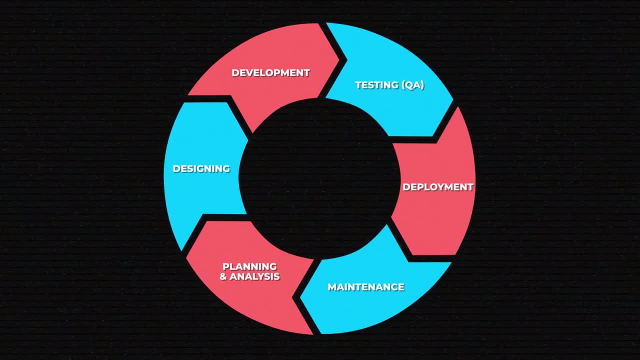 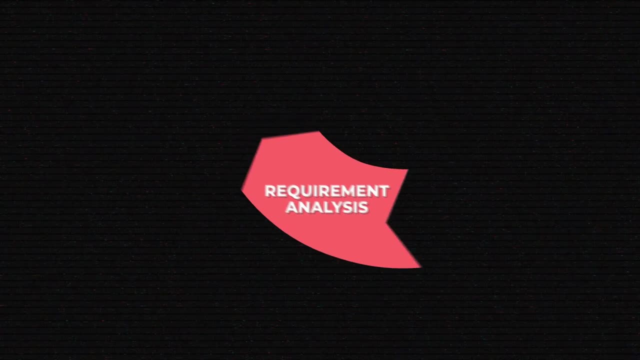 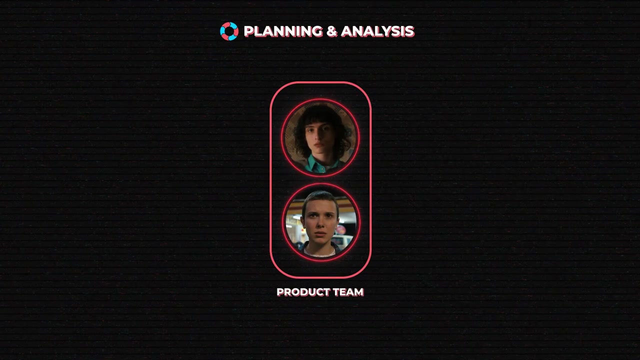 There are generally six stages of software development covered in SDLC: Planning and Analysis. It's sometimes also called Requirement Analysis or has Analysis as a separate term. Planning is a separate stage before or after planning. All in all, at this prolonged stage, the product team collects business and user requirements about what the final product must do and how it should work. 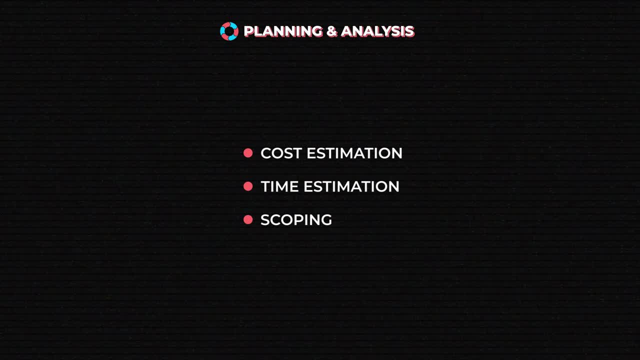 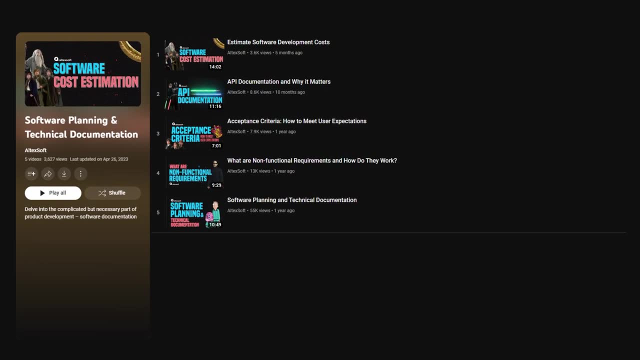 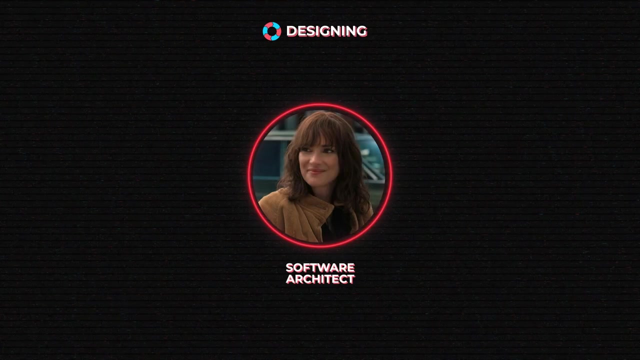 Cost and time estimation, scoping and other planning activities all go here. This is such an extensive phase that we have several videos covering software planning, so make sure to check them out. after this one: Designing: After the planning stage, you prepare the product's architecture and design. 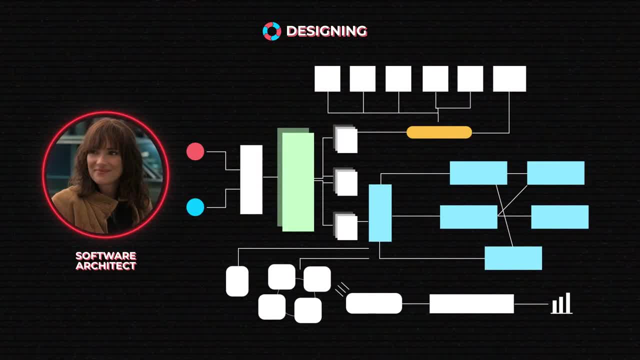 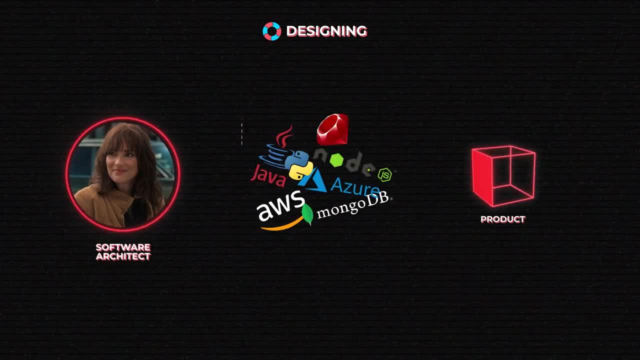 Here, a software architect analyzes the requirements and sets the high-level structure of the future systems, describing what components go where and how they interact with one another. They will also select a technology for development. User Experience and Visual Design can also be drafted at this stage. 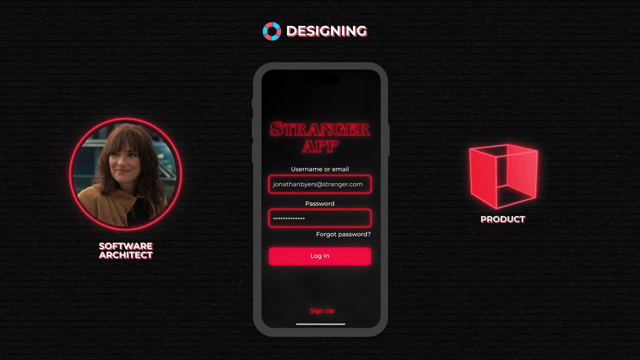 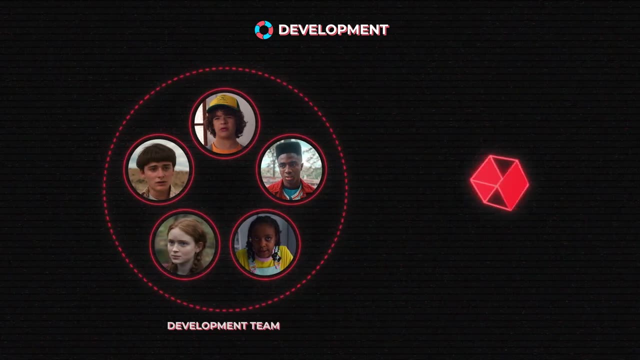 Clearly, without this stage, the following one can't happen. The next phase Development is a stage where programmers use the architect's design to write code that will finally turn the vision into reality. The next phase Development is a stage where programmers use the architect's design to write code that will finally turn the vision into reality. The next phase, Development, is a stage where programmers use the architect's design to write code that will finally turn the vision into reality. Most would understand why there are about three stages in development. The first, physics, where hardware companies as well as the software world, İt- has Virus. 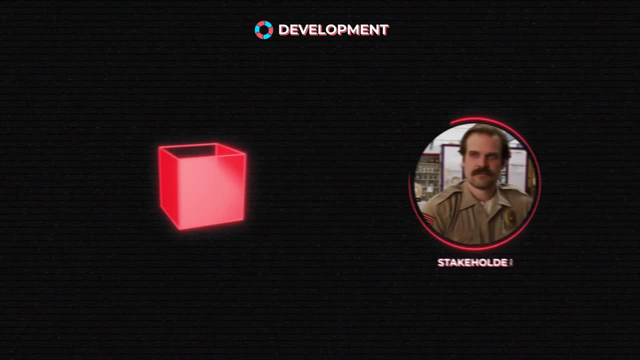 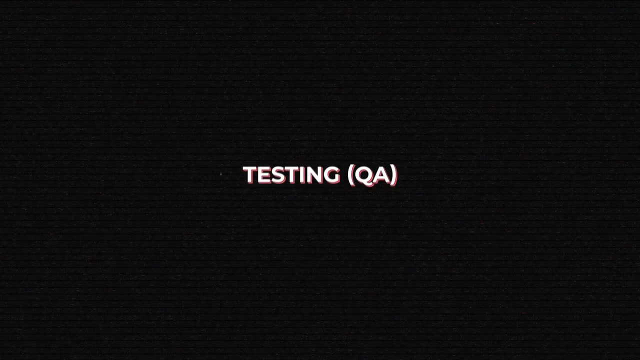 Furthermore, the next stage relies on software security. finally turn the vision into a real thing. This is where some aspects of the final product will be first revealed to stakeholders. Then testing, or quality assurance, takes place. Testers and QA professionals review the product's code. 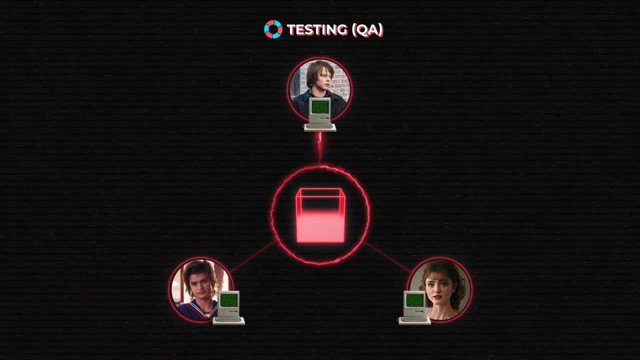 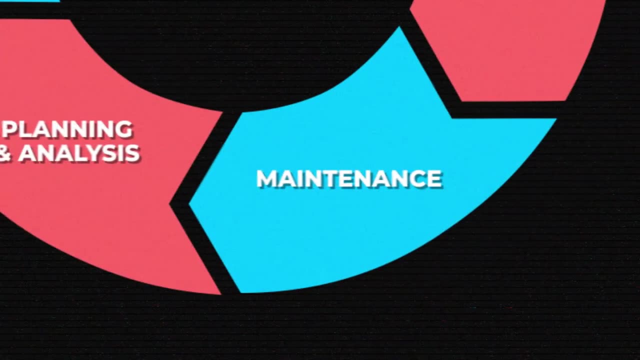 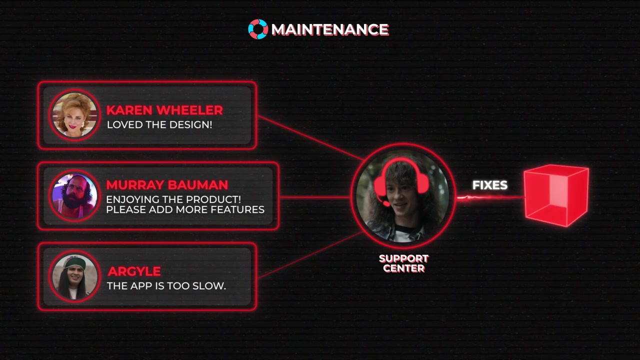 and usability, for bugs and errors, so they can be fixed before the next stage. Deployment is when the product is released to the users. Sometimes, this stage is combined with the following: one- maintenance, where feedback is constantly gathered and the product receives continuous updates and support. 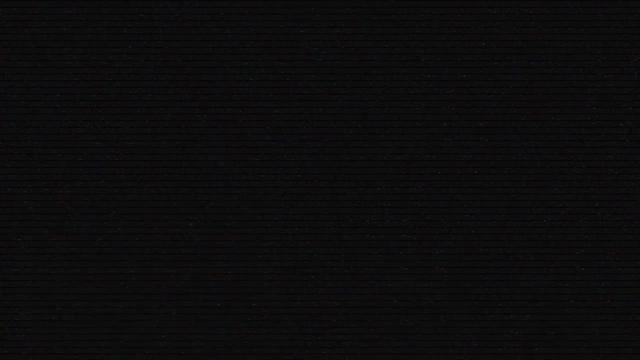 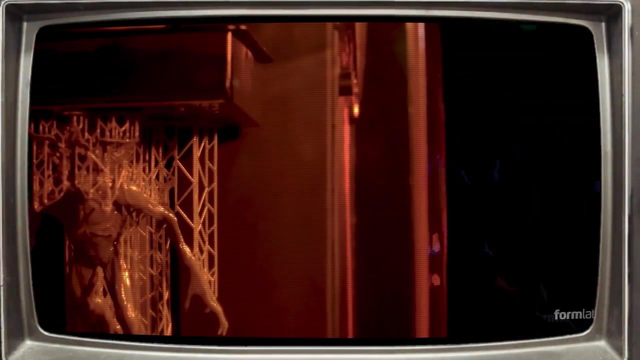 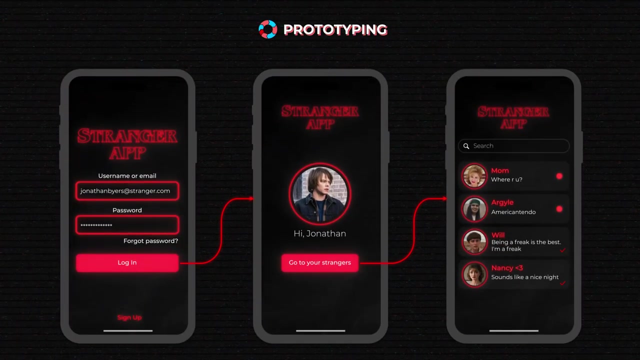 This includes both fixes and new features. Sometimes there's a prototyping stage between planning and designing. A prototype is a simplified version of the product used to validate the idea before any major work begins. It doesn't even have to be coded. The design can be used to receive feedback. 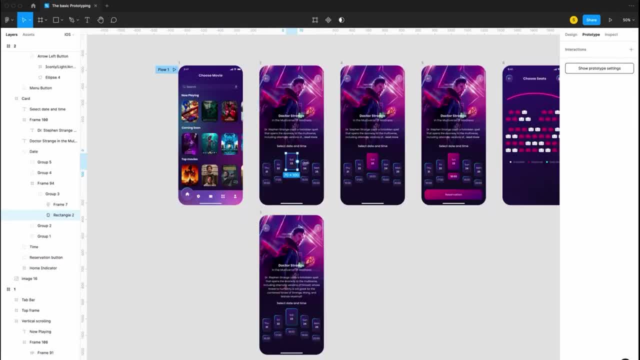 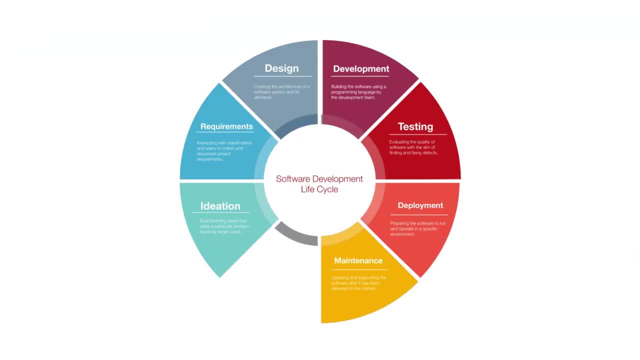 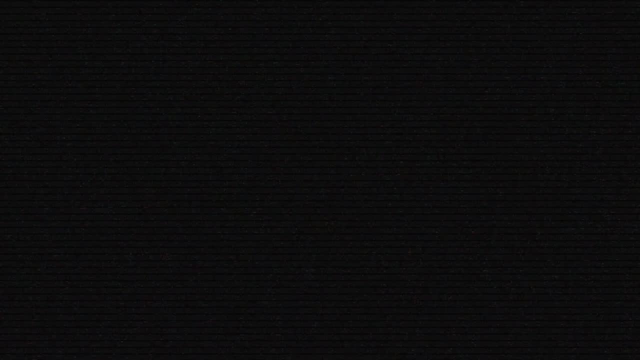 from stakeholders and users. A prototype is the best way to verify requirements with minimal effort and costs. So the number of phases and their titles can differ depending on the specifics of the projects or a particular methodology, But a common understanding remains the same. You start with a plan, then you design and develop. 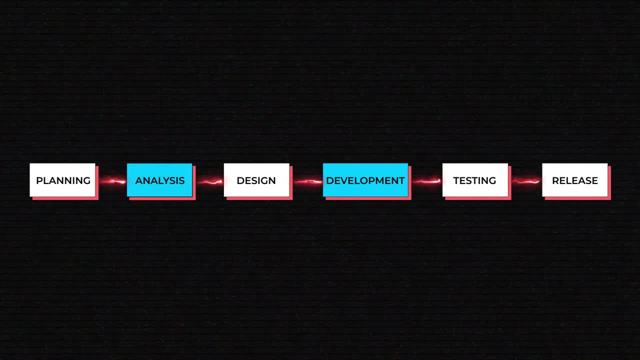 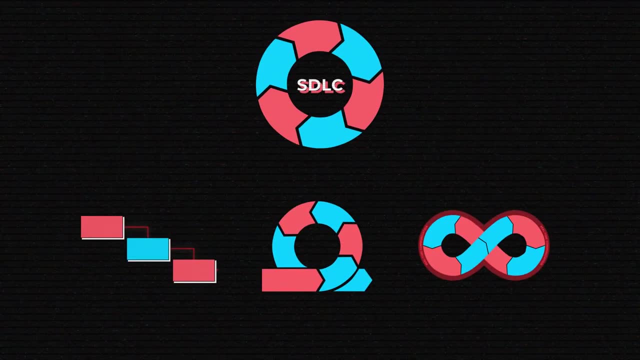 After that, you test and then release a product, But by itself, SDLC is just a concept and it's used as a base for several models you apply. that will give your project clarity and help deliver the best results. So what are they? 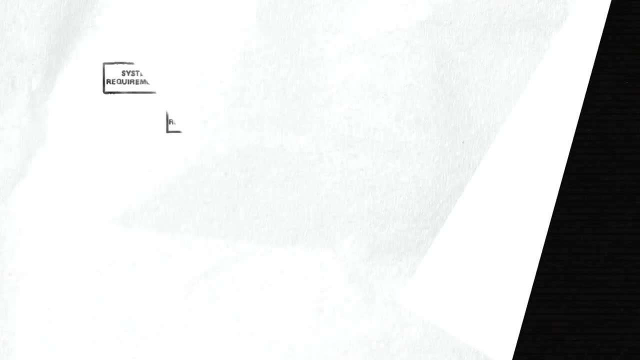 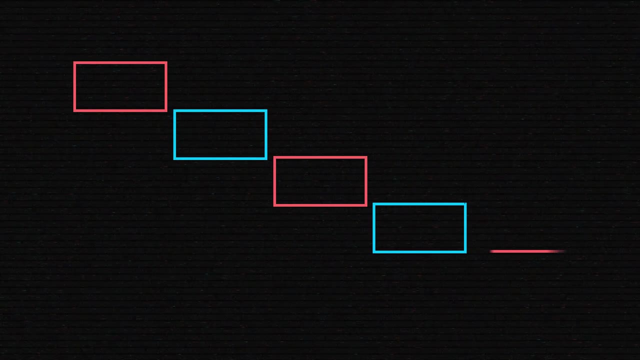 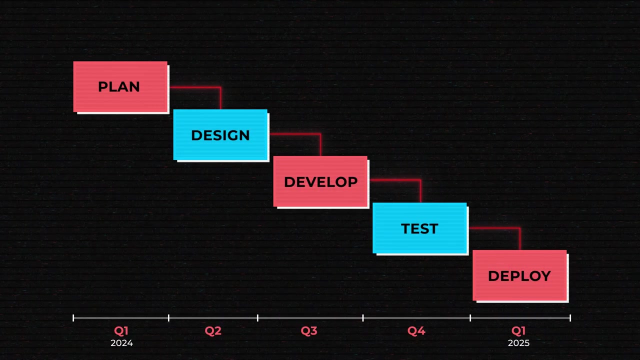 Waterfall was the first software development approach described in Royce's article back in the 1970s And it adheres strictly to the SDLC stages. The main idea is that each stage starts only after the previous one is finished. The timeline, due dates and deliverables are clearly set. 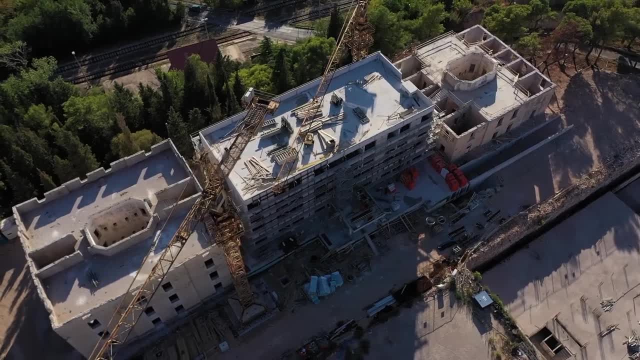 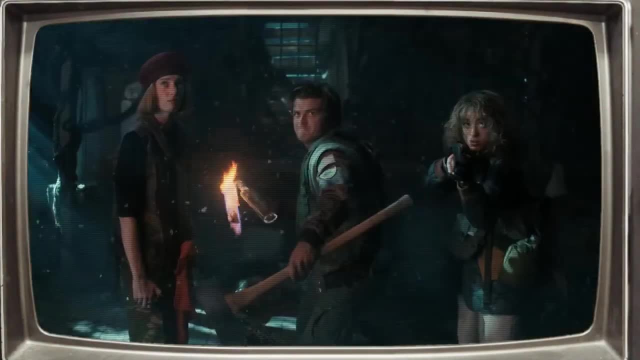 The Waterfall model was borrowed from the construction and manufacturing industries, where it makes total sense. You need to wait for the blueprints before laying any bricks. This model is very specific. It's very straightforward and well-defined, and the team can focus on just one phase. 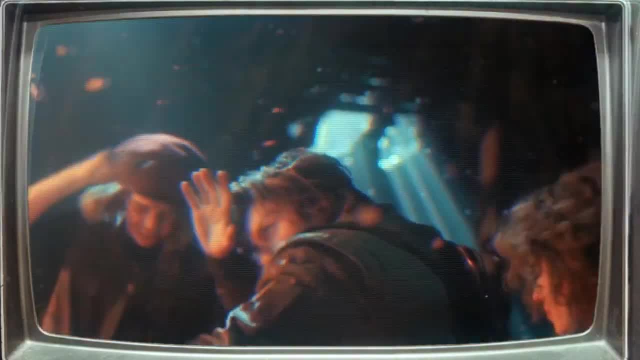 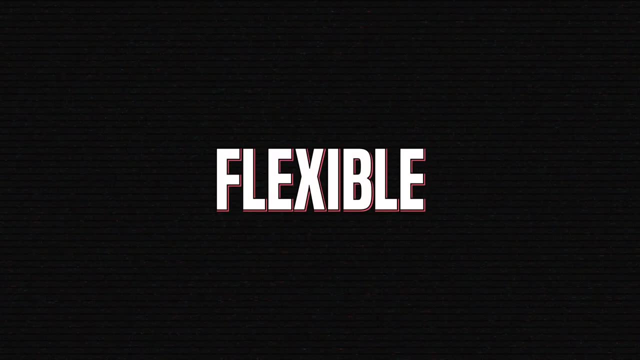 at each point in time, So the project is easier to manage. But today it's fallen out of favor in the engineering world. Why? The main reason is that it's the opposite of flexible Whenever you need to make a change in requirements or design. 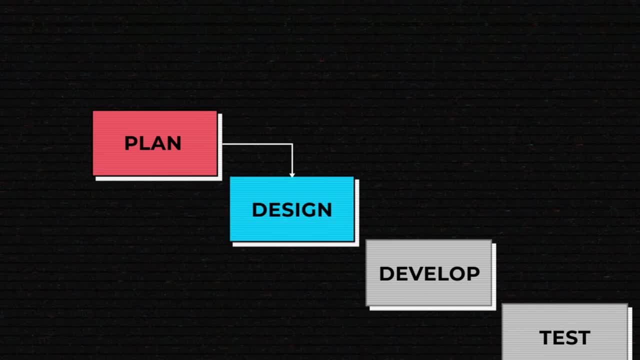 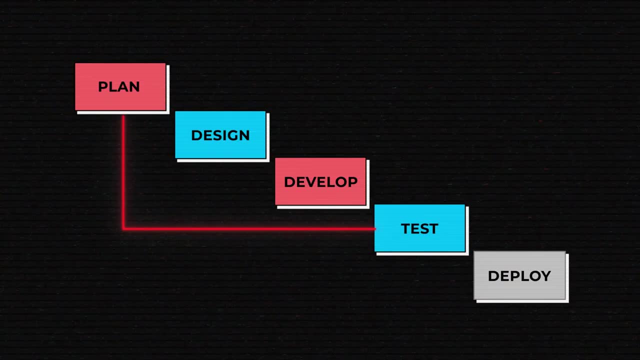 you need to roll back to stage one and do the whole cycle all over again. What if, at the finish line, you've identified some unforeseen risks that should have been mitigated during planning, If testing happens so late in the process and stages don't overlap. 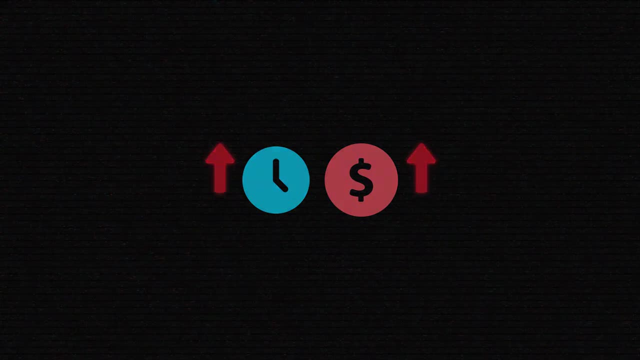 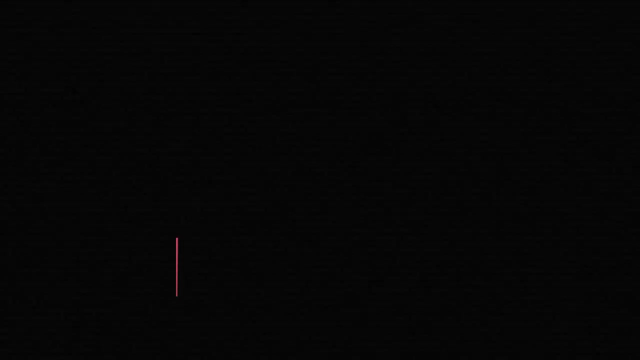 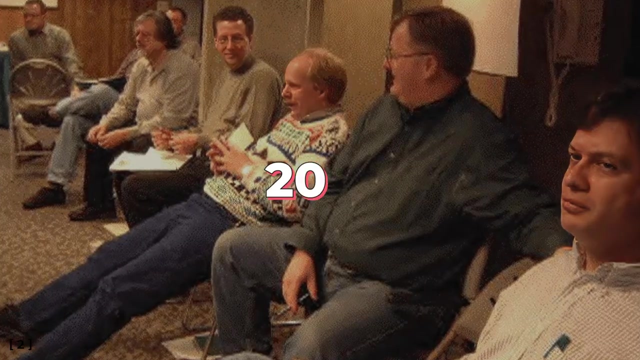 it inevitably leads to blown deadlines and budgets. So in modern software development, a different approach is used Today. agile philosophy is the king. The Agile Manifesto, which was written by 17 software developers in 2001,, was a direct response. 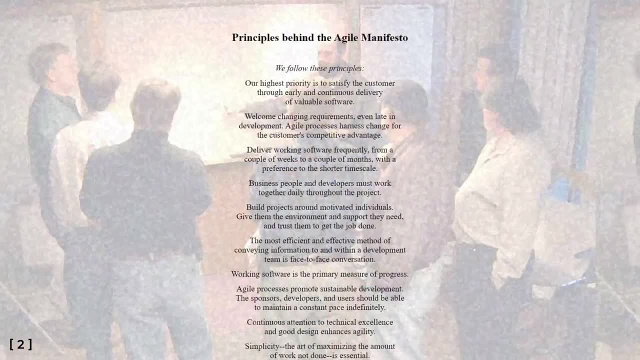 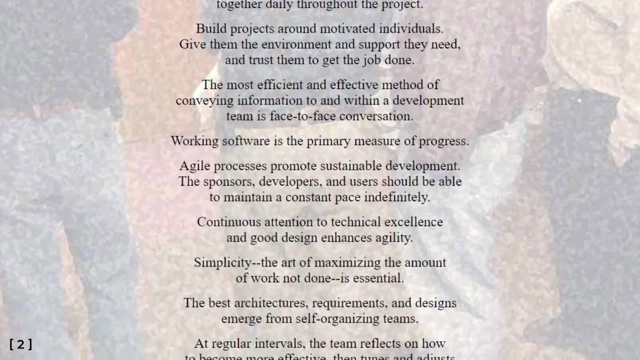 to the heavyweight waterfall methodology. Among its 12 principles, there are calls to welcome change, and it's the first step in the development of agile software. The Agile Manifesto is designed to help developers in late development stages and to deliver software continuously and early. 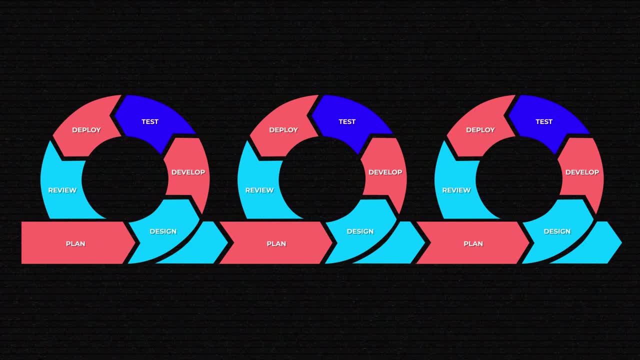 Agile solved the waterfall drawbacks in a few ways. Firstly, the testing phase isn't separate from the building phase, but rather it's done at every iteration. For example, in Scrum, one of the frameworks based on Agile, the development is broken down into smaller cycles, sprints. 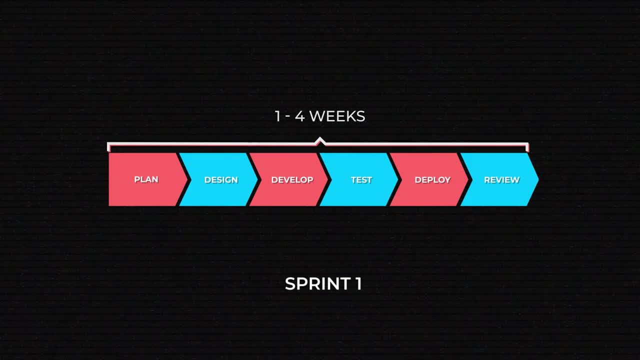 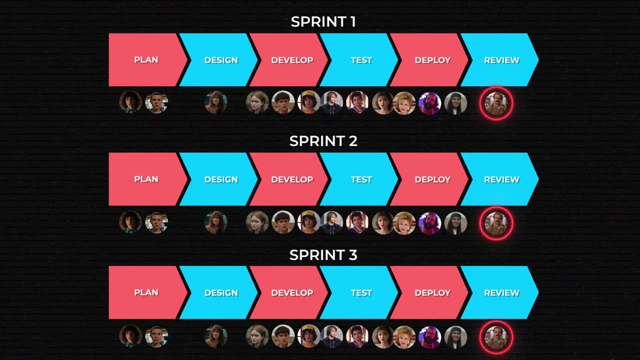 Sprints are considered to be part of the Scrum development framework, or weeks. At each sprint cycle, the team works through all stages. At the end of the sprint, the finished piece of product is shown to stakeholders. The short feedback loop allows devs to adapt quickly. 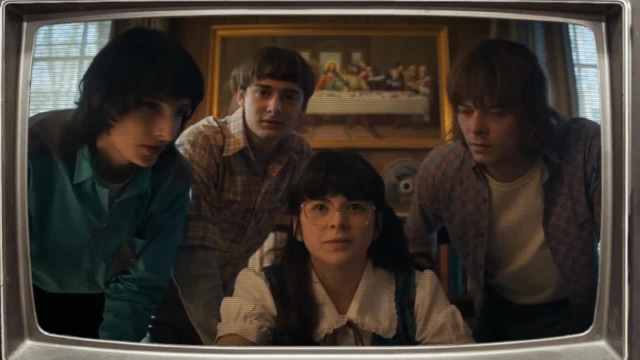 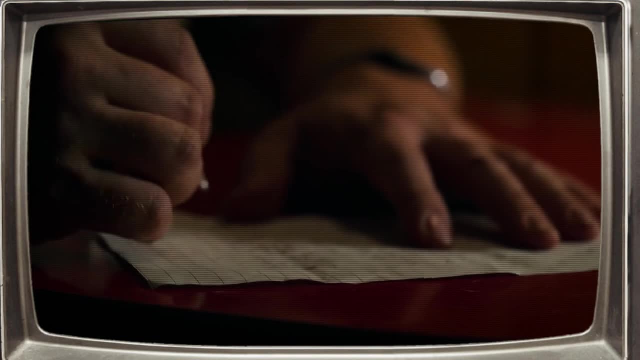 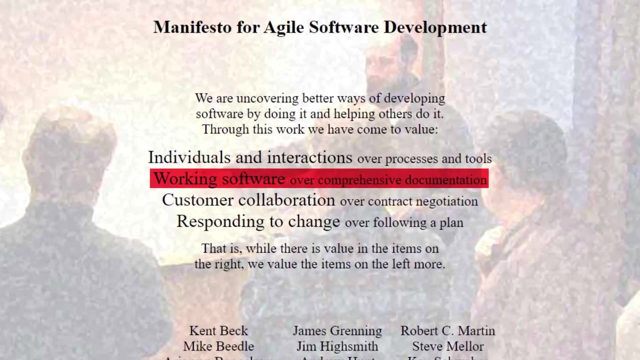 and find new approaches faster without compromising the delivery date. Another key change that Agile brought to the development lifecycle is the approach to planning or, more specifically, to documentation. One of the main values listed in the Agile Manifesto says working software over comprehensive documentation. 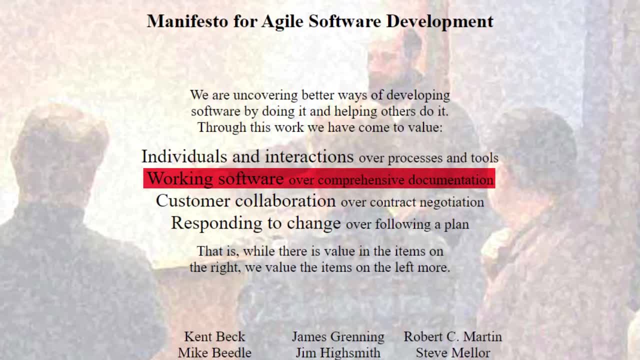 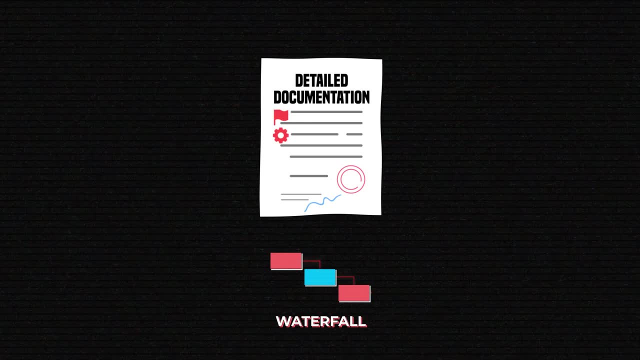 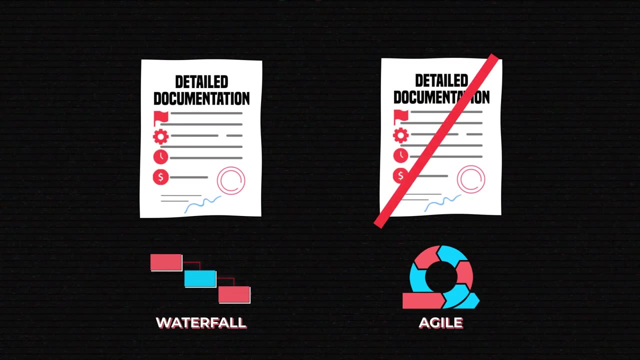 But the assumption that Agile teams use little to no docs is wrong In waterfall. the idea was to create detailed documentation covering project goals and the working process, as well as precise budgeting and time estimates For Agile, where change is welcome. this would be just a waste of time. 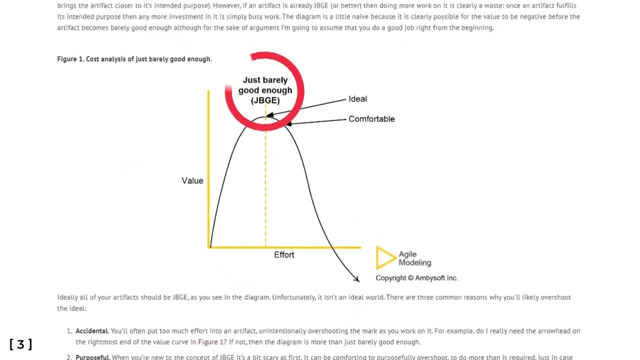 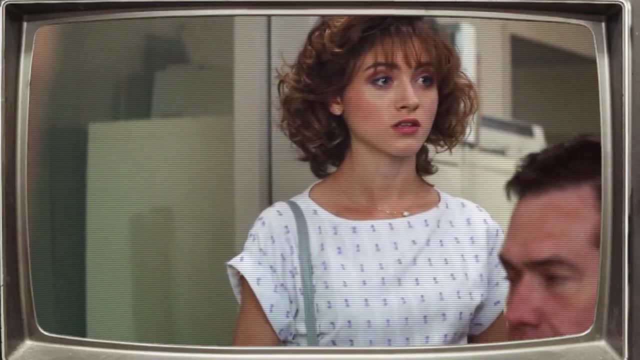 So the idea is to produce only essential docs. that is just barely good enough. Yes, this is a real term in Agile Plus. it must be a collaborative effort where a tech writer asks the team for feedback and encourages others to share their ideas. 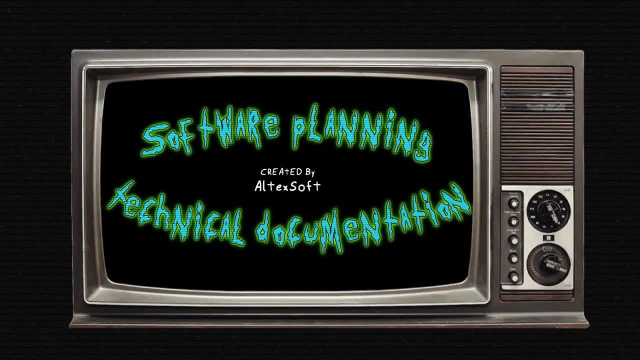 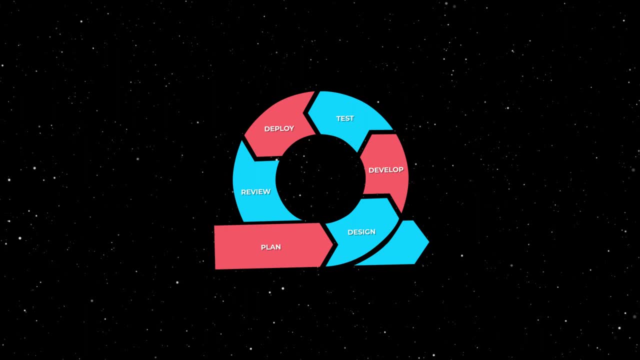 If you want to learn more about documentation types and how they're created, we have a few videos you'll find useful. While originally Agile was more of a philosophy, today it has loads of specific tools and techniques, Such frameworks as Scrum, Lean, Extreme Programming. 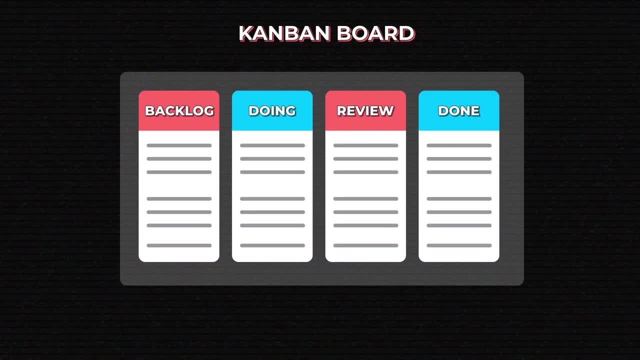 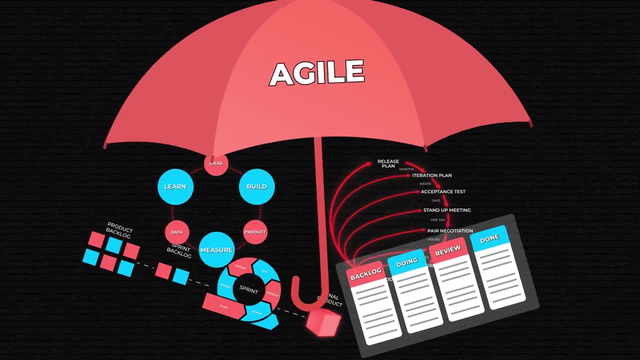 or Kanban are also classified as Agile approaches, even though they existed before the Agile Manifesto was formulated in the first place. Now that they've been implemented, they now fall under the Agile umbrella. Each framework has its best applications and specific toolset. 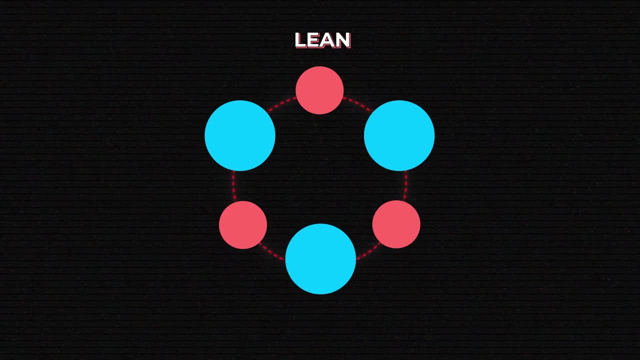 Apart from the aforementioned Scrum, there's a Lean methodology that focuses on eliminating waste and at its core is a feedback loop for testing your assumptions. It consists of three recurrent steps: Build, which basically means drafting some version of the product, such as an MVP. 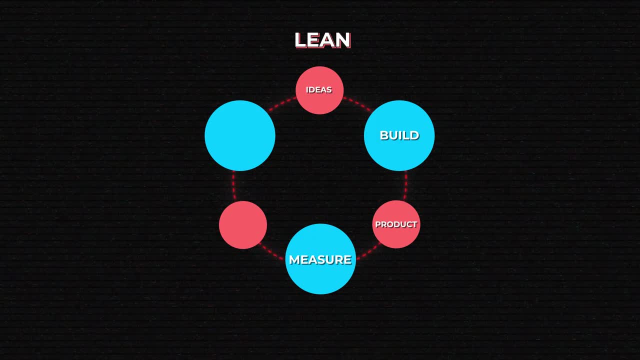 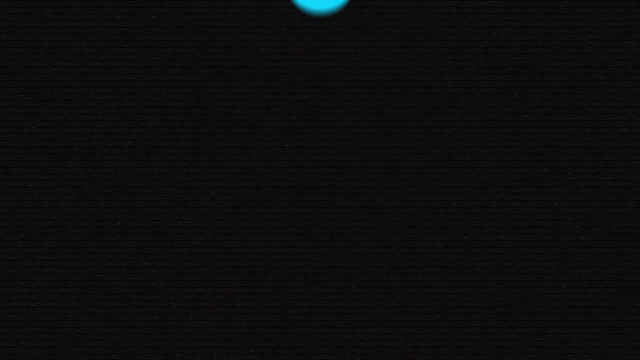 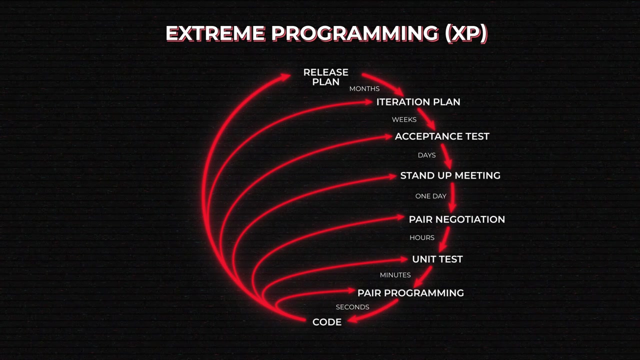 Measure, meaning collecting feedback and evaluating if this version of the product succeeds And learn, drawing conclusions and deciding how you'll refine your product for the next loop. Another framework called Extreme Programming or XP uses the usual lifecycle but emphasizes the technical aspect of development. 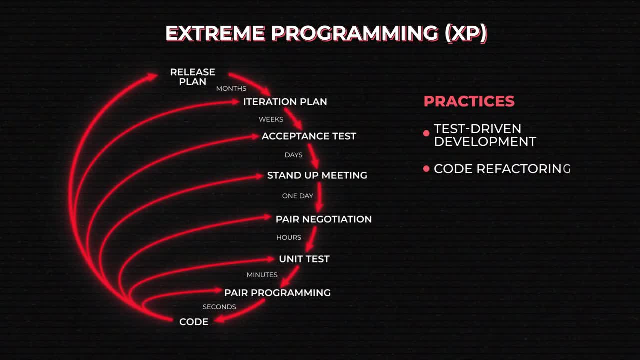 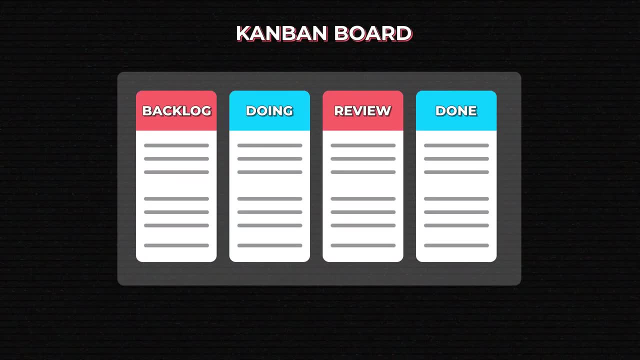 It uses such practices as test-driven development, code refactoring, pair programming and more. Also, Kanban is more of a management method than a framework, since it uses so-called Kanban boards to visualize work for efficiency. There are many more frameworks in the Agile world. 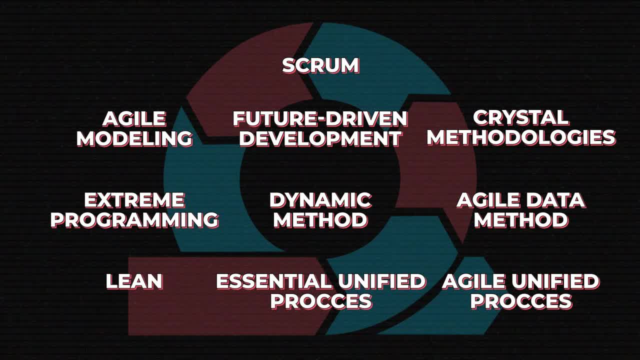 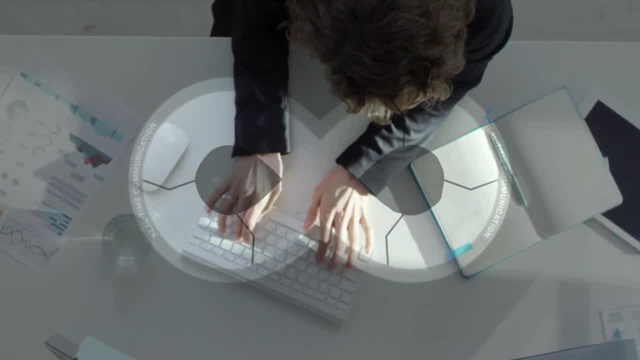 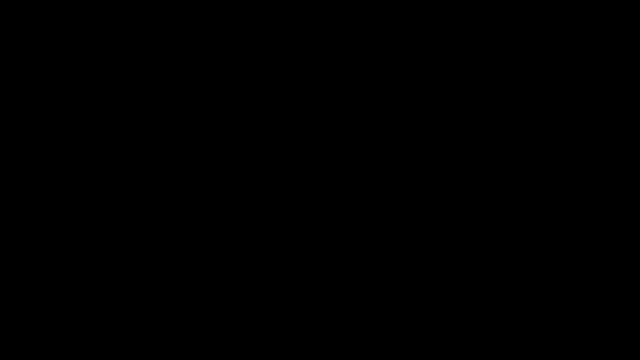 including the Agile development process that can be used depending on what the team wants or the project requires. Around 2008, a new concept emerged from Agile that drastically changed how software is built and released. today, DevOps is one of the most discussed development approaches. 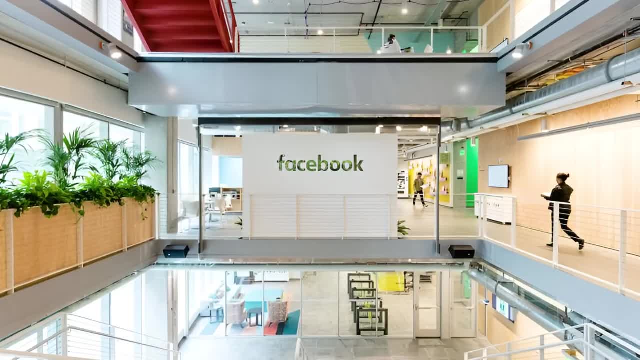 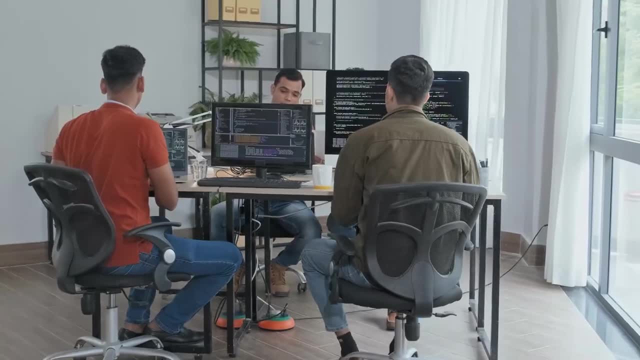 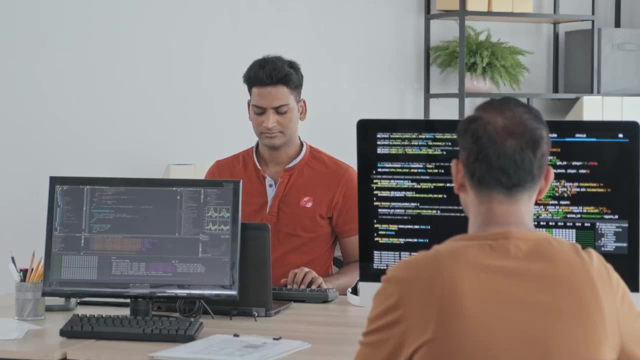 employed by such giants as Amazon, Netflix, Google and Facebook. It stands for Development and Operations. DevOps introduces a cultural shift where different teams work together. Developers, QAs and operations are no longer writing the code, testing it and deploying and supporting the code apart from one another. 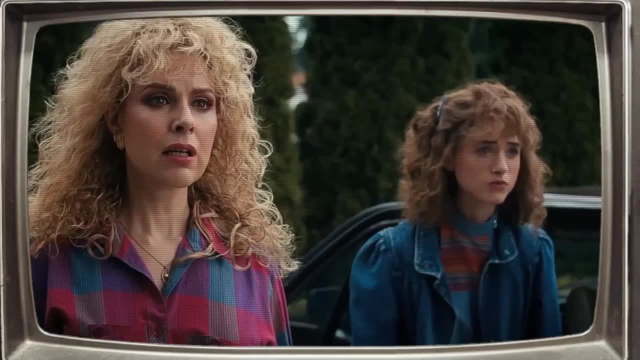 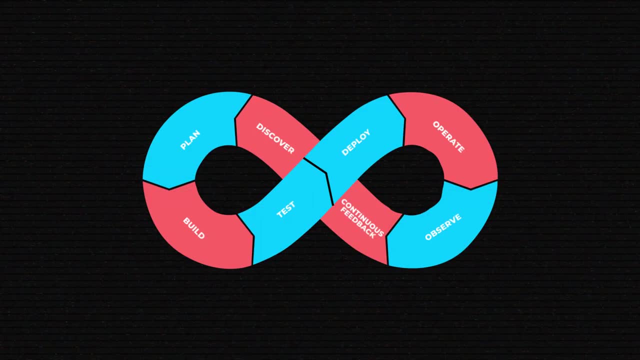 Now they merge into a single team, often having multidisciplinary skills. DevOps' lifecycle is typically visualized as an infinity loop, representing the development processes on the left side and operations on the right side. A team collaborates and communicates throughout each phase. 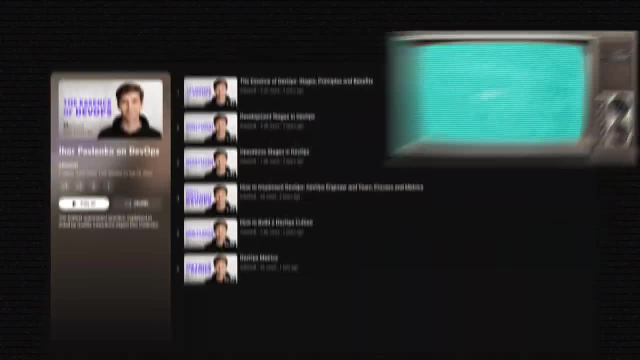 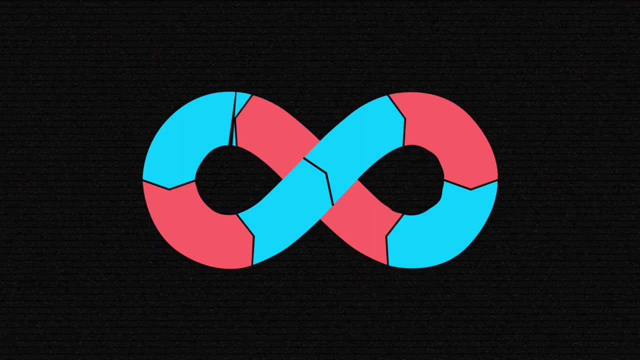 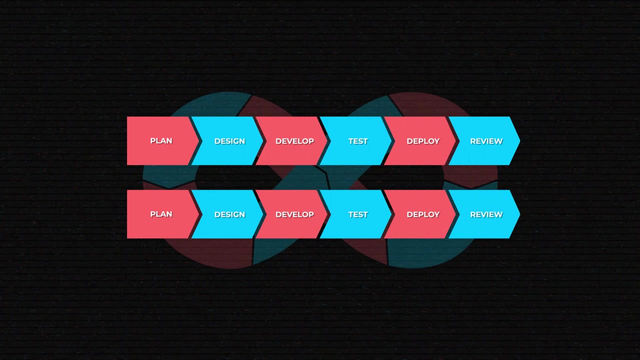 We have a whole separate video covering DevOps and a video series about all DevOps aspects you need to know, so check it out after this one. What's important is that DevOps uses typical Agile planning. The product development has rough objectives outlined and only the few future sprints are detailed. 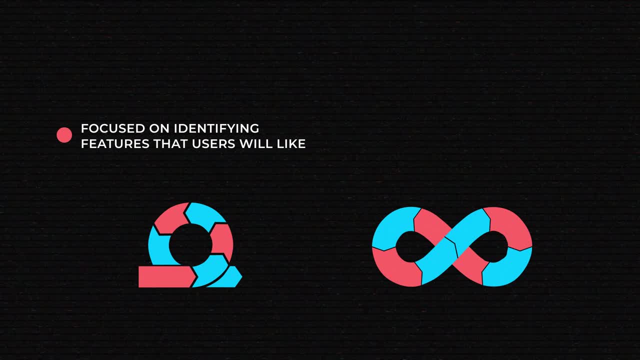 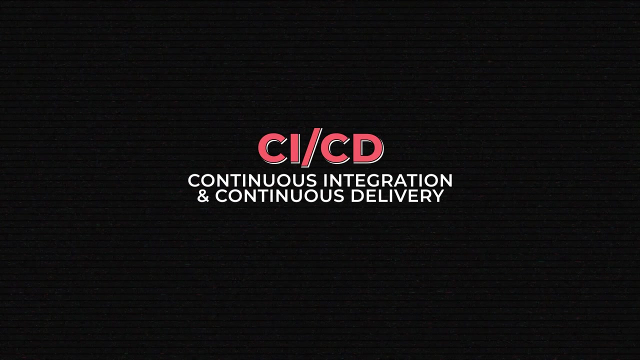 So, while Agile is focused on identifying features that users will like, DevOps makes sure that existing processes are optimized and streamlined. To do that, DevOps uses CI-CD- Continuous Integration and Continuous Delivery- or CI-CD, is a set of principles that allow developers to deliver frequent code changes. 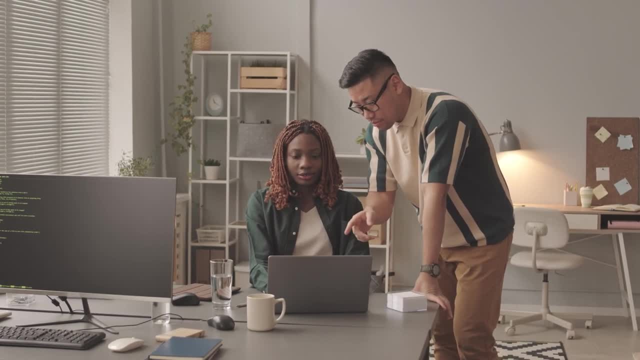 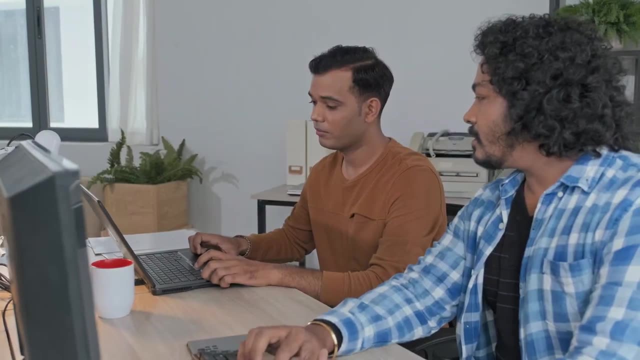 It means that teams integrate code on a daily or even hourly basis by merging code changes in a central repository and preparing for deployment at any moment. Basically, all changes, new features and bug fixes are always ready to be deployed and the product can be updated multiple times. 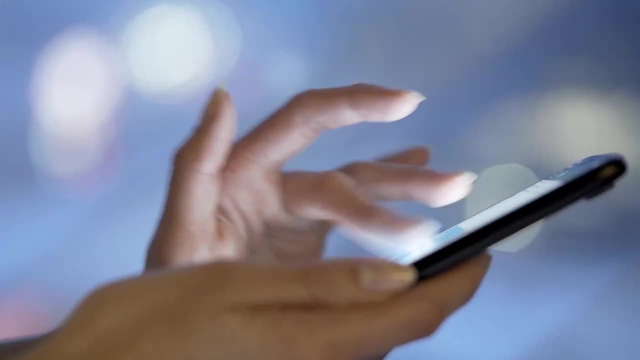 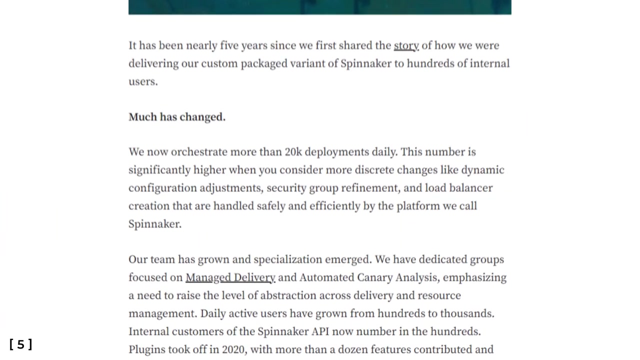 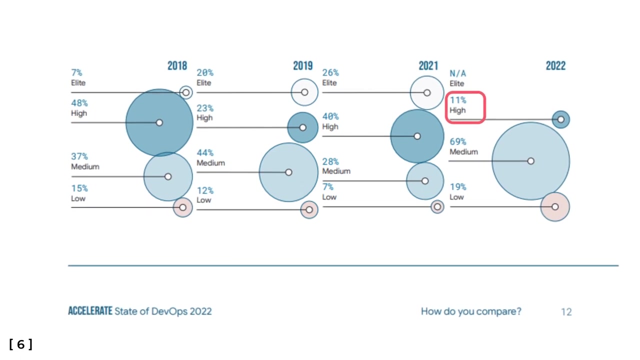 Continuously delivering value to users. HubSpot shared that they add 200 to 300 deployments a day using CI-CD. Netflix orchestrates over 20,000 deployments daily. In 2022, 11% of organizations were considered high DevOps performers. 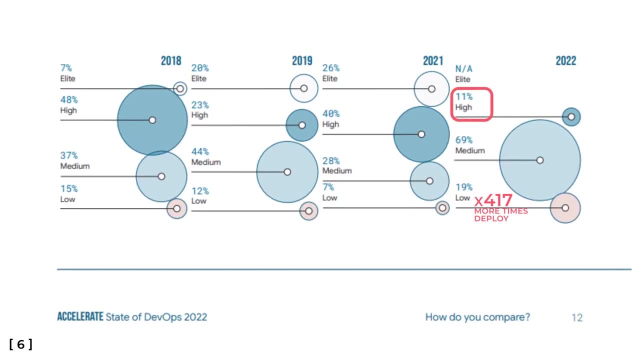 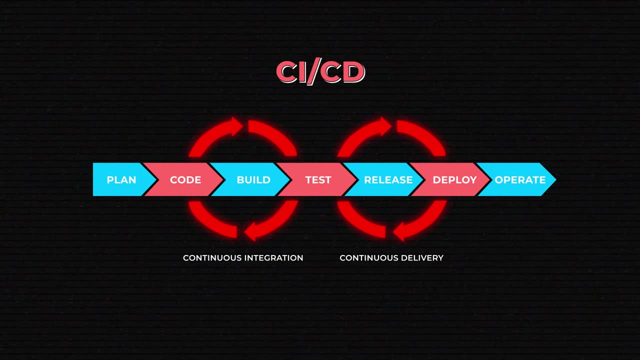 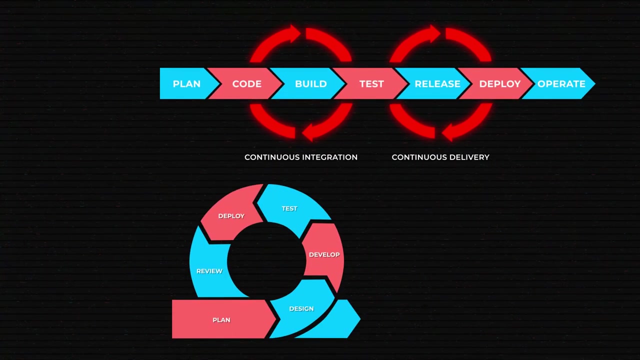 and deployed 417 more times than low performers. This is, of course, achieved by high levels of automation and the infrastructure that connects all aspects of product delivery and a unified ecosystem. Although CI-CD facilitates agile practices such as getting feedback quickly and detecting errors in the early stages, 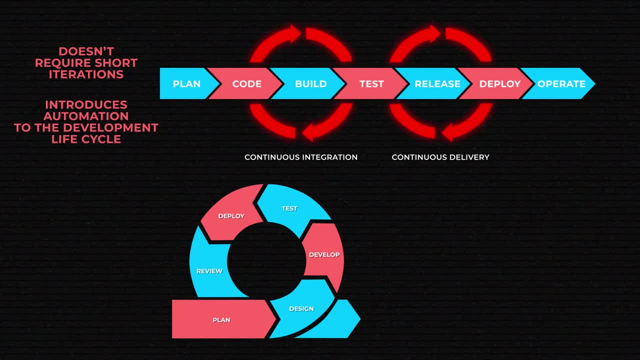 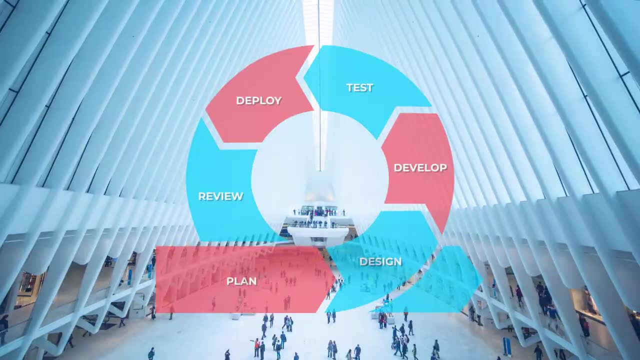 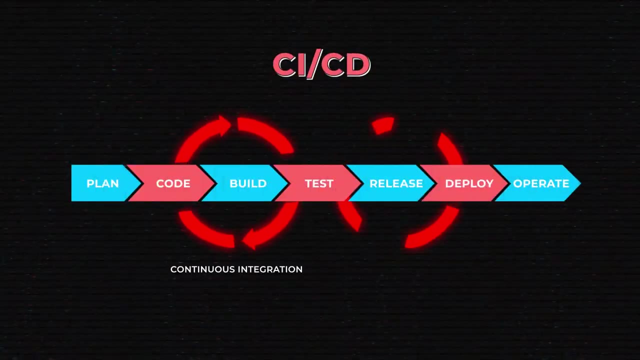 it doesn't require short iterations and introduces automation to the development lifecycle. Even in agile, introducing product changes can be a long process, especially today, when technological innovations happen so fast and consumer needs change easily. So CI-CD solves this problem by adapting in a short amount of time.